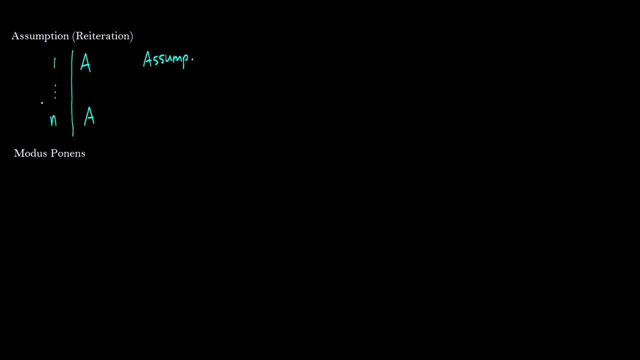 we want. so say, if we have an a at line one, we can rewrite it again at line n. This just means from anywhere And we write one re-it because we have to remind ourselves what we did on each line. so that way it's true And we have justification of what we did. So what this? 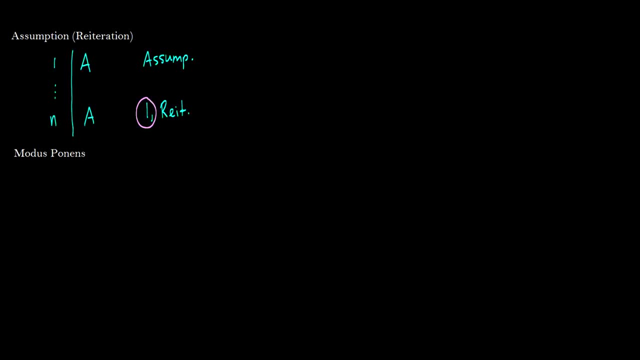 means is that from line one. we reiterated it. So this is one of our basic rules. Another one: here we have a thing called modus opponents, and you might remember this. If we start off with, say, on line i we have a, On some other line we have a arrow b, Then we can conclude b from. 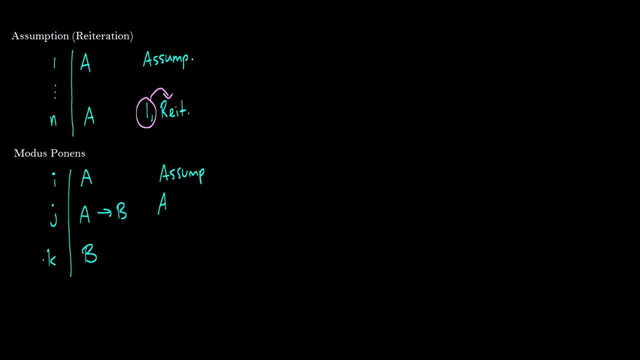 well, let's call these assumptions. So this is an assumption. this is an assumption. Then b we say, is from line i and line j and this is mp for modus opponents. Now, when I say line i and line j, I just mean any line. If it's a, two and a four, there you just put two, four mp. So this is also. 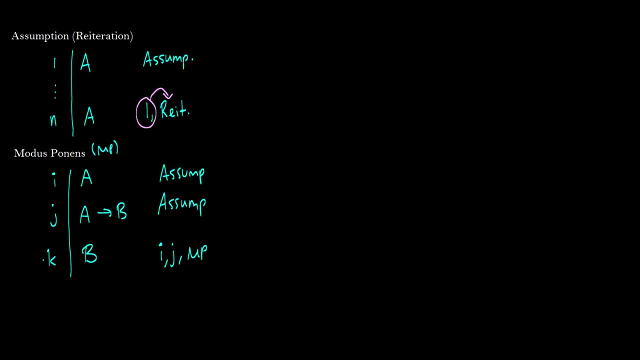 called conditional elimination sometimes, which you might see as that. This is a really weird term for this because it's modus opponents and it is a conditional elimination, And then we have commonly used term everywhere in philosophy. So I kind of can question books that use arrow. 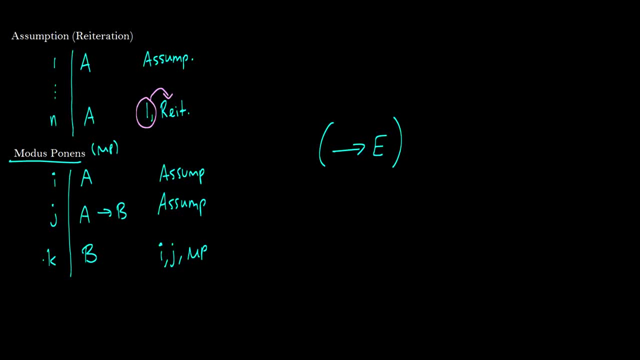 elimination, or they call it conditional elimination. It's kind of weird, It bothers me in ways that it shouldn't. And elimination- Okay, here's another good one. We also abbreviate this like this: If you have a and b on some line, then later you can get, and It's just a, You can. 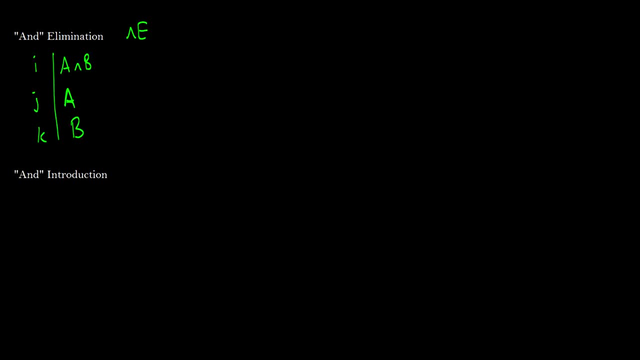 get any one of the disjuncts you want, So you can get a or you can get b from it. Well, you get both, but you can. you have to write them down separately. So we'd say: this is i for, and elimination And. 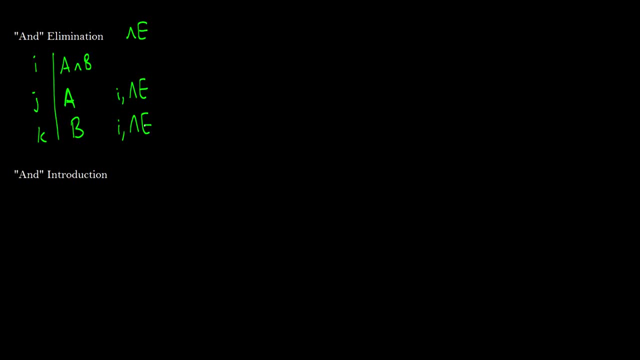 this also comes from line i for and elimination. So this is an acceptable rule here, And introduction states that if you have three lines- i, j and k- if you have a on one line and b on another line, you can put them together to get a and b. So we have i and j And this is an introduction. So 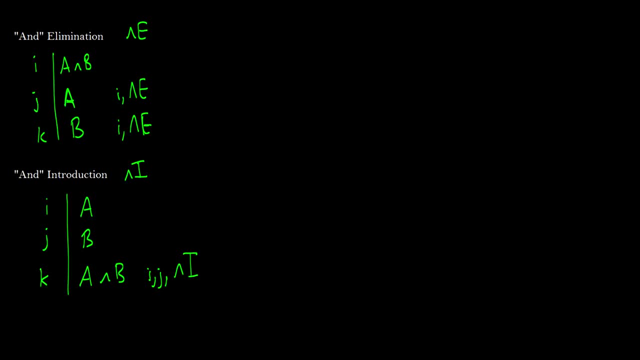 every elimination rule has an introduction rule. So this is the opposite. So if you have a and b, then you can get a and b. And finally, some last rules we're going to do today is: or introduction: If you have on line i some statement p, then on line j you can write p or anything, And this: 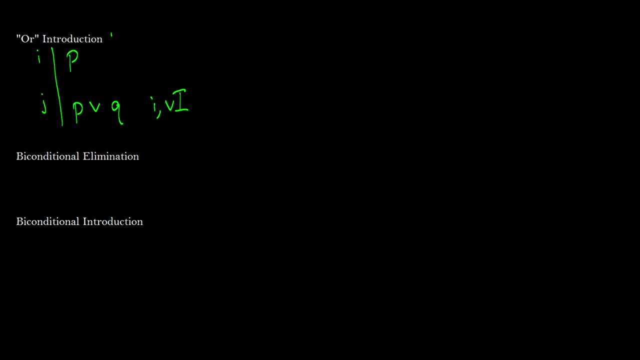 comes from i, and this is- or introduction Or elimination- is very difficult, so we're not going to do it in this video. But if you take a look at this, this line says that p is true. So we know that disjunctions are true if at least one of its disjuncts are true. So p is going to be true. So 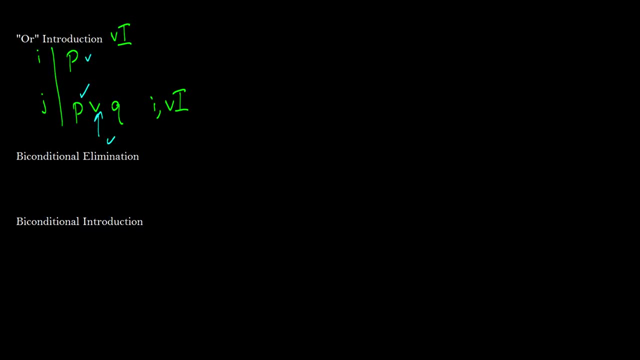 since it happened in this instance, it's also going to be true, no matter what you put there. So it's totally acceptable. Biconditional elimination is sort of a tricky one. If we have a biconditional b, then what we really get is a-arrow b and b-arrow a And biconditional. 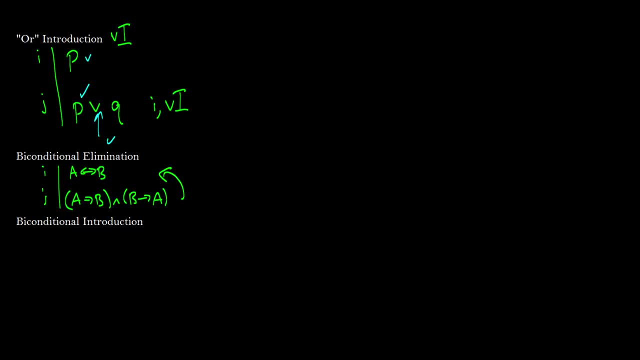 introduction is really just the opposite way. So them like this: elimination and introduction. these aren't rules you commonly use. in fact, one given in the logic book that I like is that if you have a arrow, double arrow, B, and you have a, then you get B, and I like this because 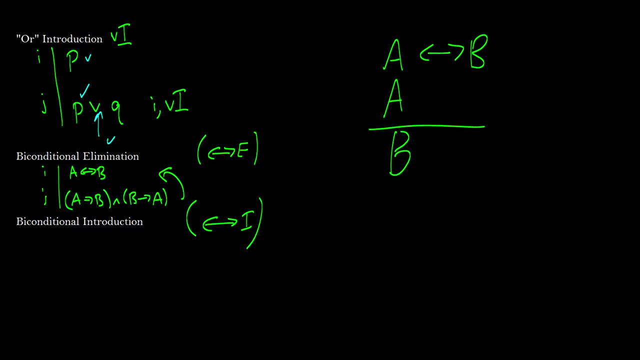 both the truth values have to be exactly the same, so this is also going to be acceptable for us. similarly, if you have a by conditional B and you have not any, then you're gonna get not B, because the sign must be the same for both of these. 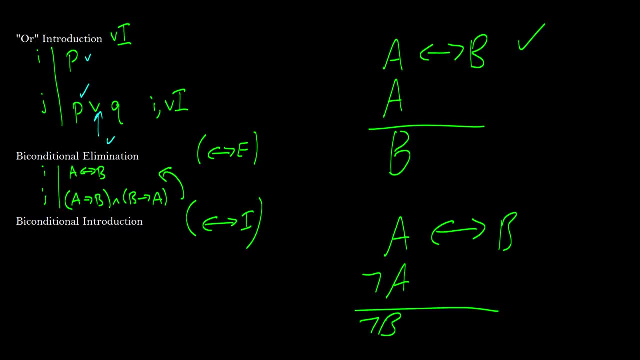 and this is fine for me. you can call this by conditional elimination. depending on your class, you might have to use specifically one of these, but for this video series I'm just going to be using both interchangeably. they're both proven from each other, so it's not really necessary that I 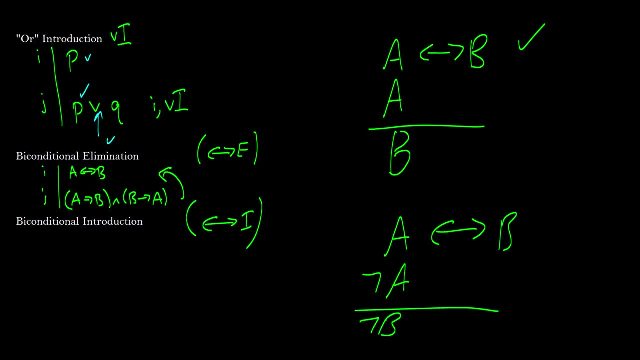 put them in the same order. so I'm just going to put them in the same order. so pick one or the other, because both of them are valid. it's just depending on your professor. you might have to prove one or the other. all right, let's do some. 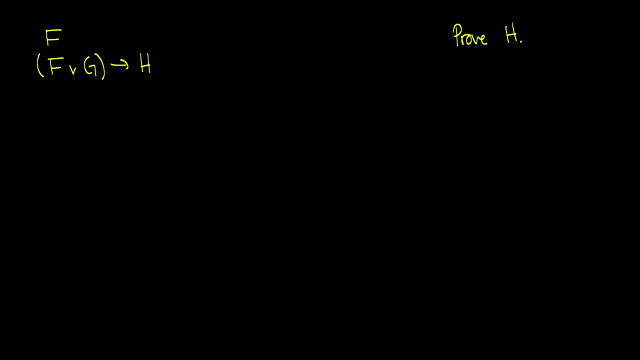 examples: we're given F and F or G, arrow H and we have to prove H. so let's set this up Fitch style. so we put a line on the left side, we number our lines and we have to a label each of our lines as justification of why it's. 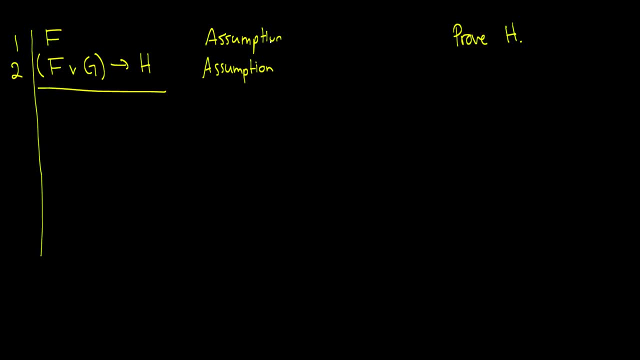 there, because if we can't write why it's there, then why are we writing it? okay, so what's the first thing we can do? we're trying to get to H. so we take a look at what can possibly get us to H and we see this line here: F or G, arrow H. so we know. 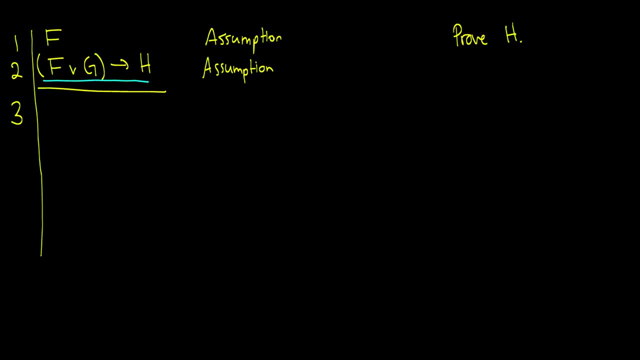 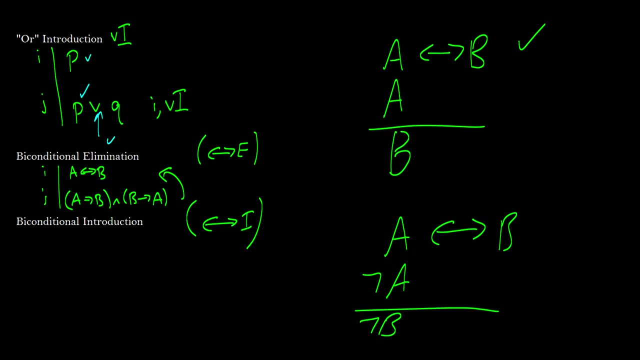 we need to get an F or G in there. so what are we going to do? well, we use an rule we have with F, so we take F from the first line and we just add, or, so on one we use, or introduction, which is going to be this rule, right? 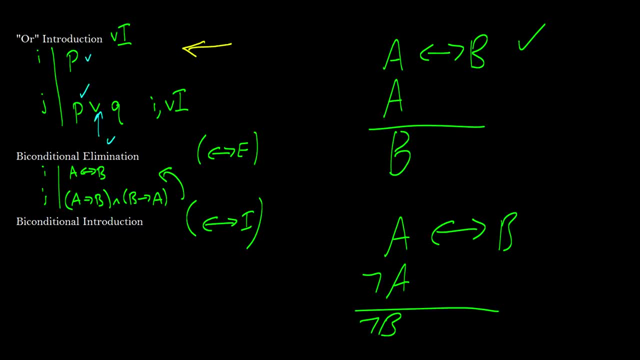 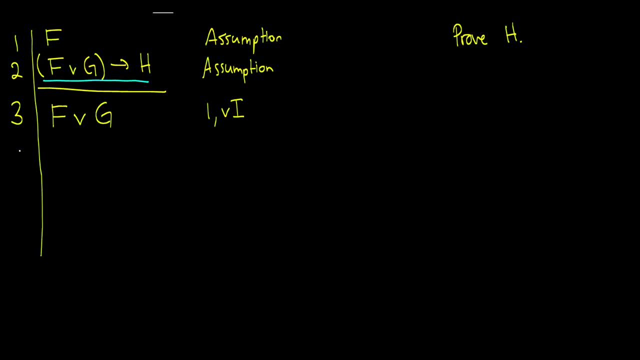 here, if we have P on one line, then on another line we can put P or Q and those can be any letters you want. so that is the first step. and on line four: well, we know we have a rule called modus ponens that if we have F or G then we get H. we 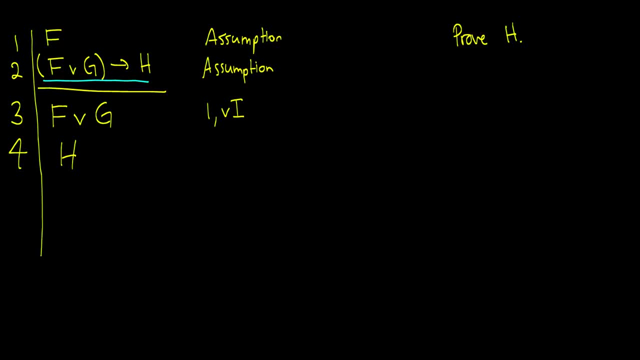 have F or G, therefore we get H. so this would be lines two and three, modus ponens, and this is the end of the proof. so we have proved H from it. all right, let's try another one a little bit harder. so with these two we want to prove not A and B or C. so this is a. 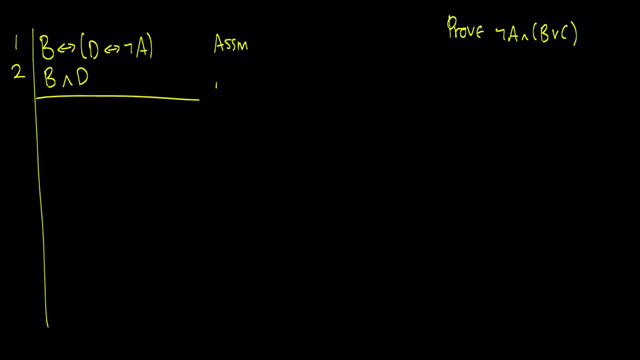 little bit crazy. I'm just gonna write ASSUM on the top. I'd shorten it further, but I think that's fine. I'm just gonna write ASSUM on the top. I'd shorten it further, but I think that's fine. I'm just gonna write ASSUM on the top. I'd shorten it further, but I think that's fine. 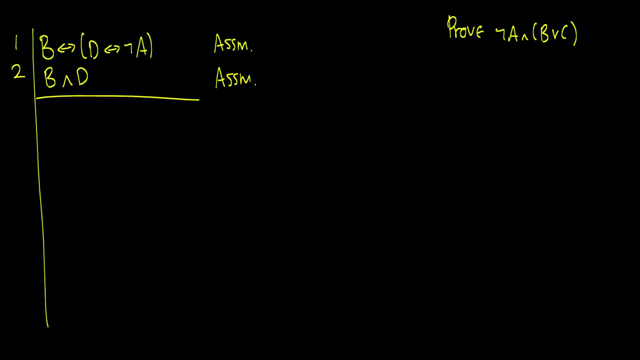 for a YouTube tutorial. I'm gonna refrain from that. you might be able to guess why. so here's what we have. we have B biconditional, D, biconditional, not A, and we have B and D. so let's use AND elimination first to get B and D on. 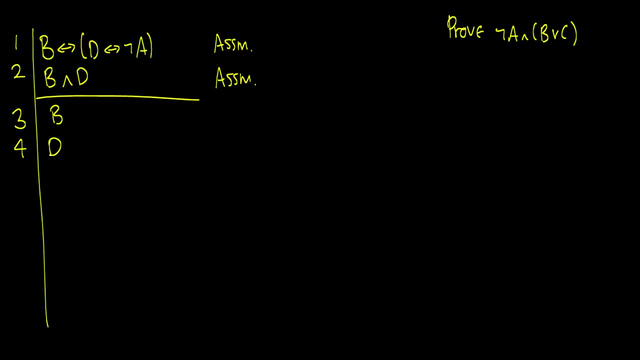 their own, because it's usually good to separate everything you can so you can see what you can do with it. so this is gonna be: AND elimination on two, and this is gonna be- AND elimination on two, and this is gonna be- AND elimination on two and this is gonna be. 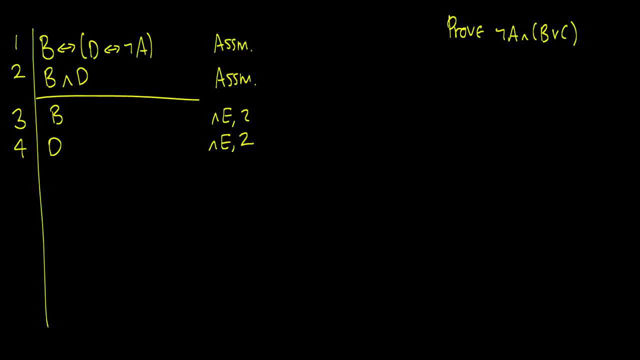 AND elimination on two. now we have B biconditional, D biconditional A. so with one and three, we know that if B is true, then D biconditional, not A has to be true as well. so we're gonna call this biconditional elimination and we also 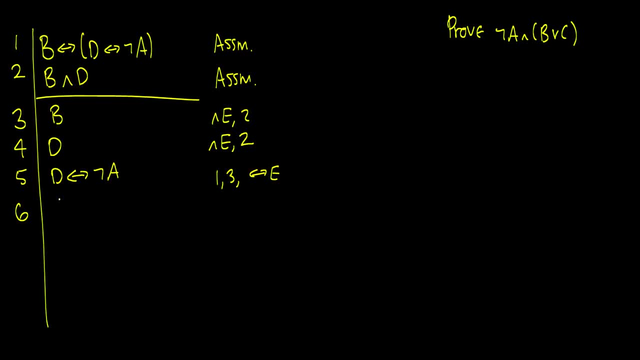 have D true, which means that not A has to be true, using four and five biconditional elimination. so now we have not A, but we have to prove not A and B or C. so we have our not A. now we just need to get our B or C. how do we do that? well, 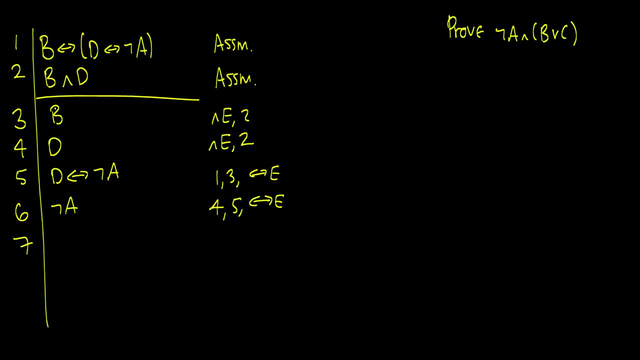 we'll take a look at line number three, where we have B and we can use OR introduction to get B or C, because that is a rule and we are allowed to do that. and now on line eight, we can conjoin the two using AND introduction, so we get not A AND B or C. 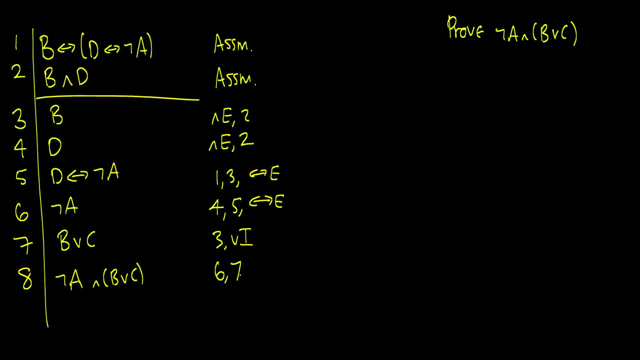 so this is lines six and seven with AND introduction. so I know this might have been really fast if this was the first time you've ever seen this stuff, because the rules came fast and furious and I definitely beg of you to do a bunch of practice, because practice is going to be the best thing you can do to learn these. 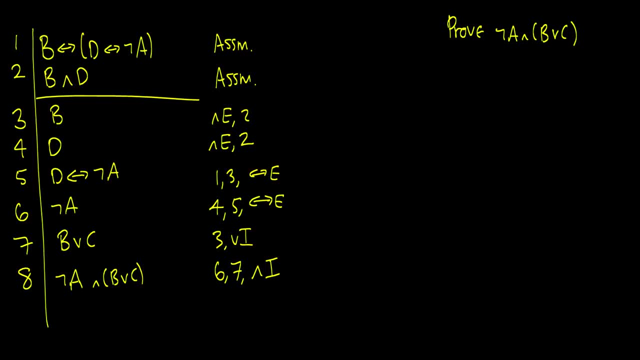 rules. so I'm gonna give you a bunch of practice questions that you need to do. I'm not giving answers- I'm not going to do answers for these because they do take a little bit- but by doing this you should be fine to do the next thing. 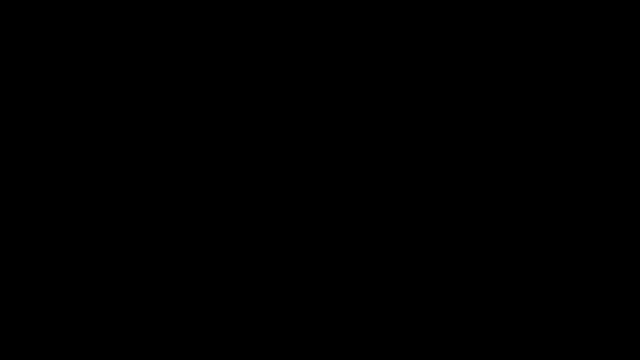 and you should get it. if you have any questions about the proofs I'm gonna give you- they might be difficult. okay, they might be difficult. if you have any questions about them, please leave them in the comments. I will answer the questions about these proofs because when you practice them and you get to, 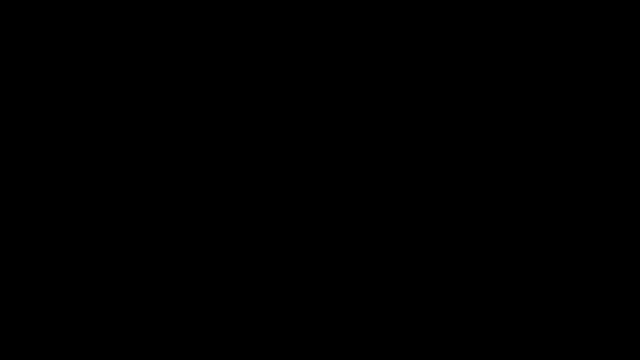 know them, these become very simple, but at first I know they're incredibly daunting, so I need to let you loose on your own to try these, okay? so I know you don't want to, but you have to do it. so here we're given A arrow B and not C. we are given A and B and I want you to prove not C. this one should. 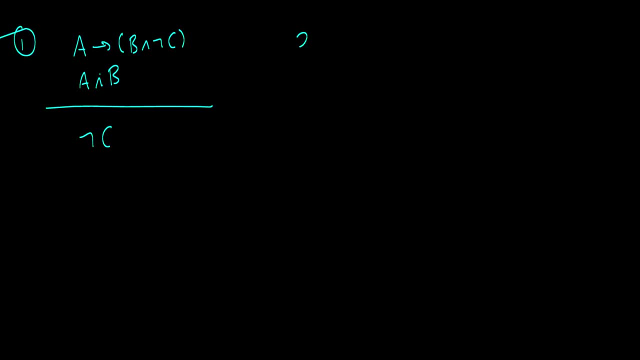 be a little bit simpler for number two. we are going to do not B arrow D and E. we're also going to give you A and not B and C, and we want you to prove that. you, I do believe that this one is pretty easy and we wanna do it. but I also want 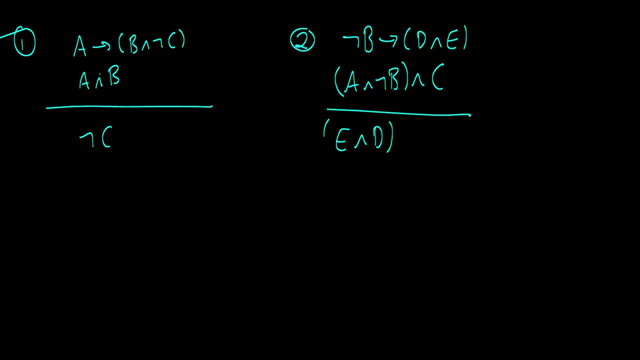 you to prove E and D and not B and C, even though it does not really go the way. Let's give you a few more because I do believe that practice is amazing. so let's give you a few more because I do believe that practice is amazing. so. 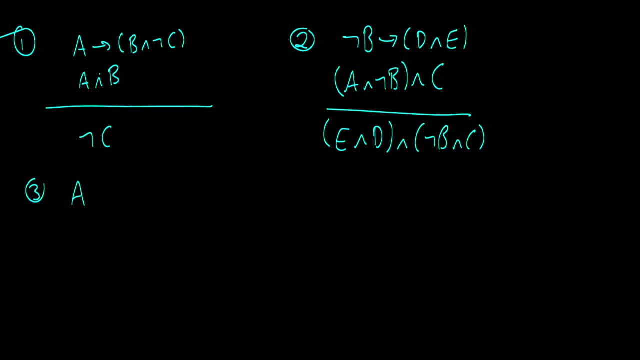 here's a nice hard one, okay, so for number three, we're going to do A and not B, and A or not C arrow D, and we are going to prove the freedom that the. what are we going to prove from this? Let's do this real quick: We can get D and we can get not. 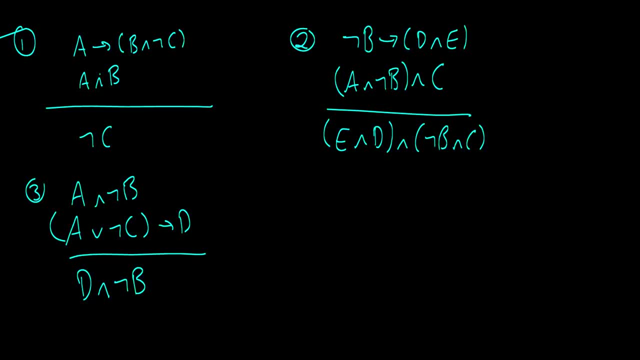 B. That should be provable. And finally, let's give you a three-liner, for what can we do here with this one? Okay, we'll get not F and not G, Not G arrow. H, H and not F is biconditionally. 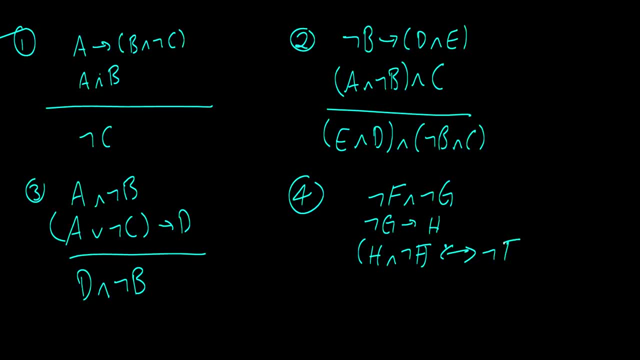 equivalent to not I, And from this it should be very easy to get H and not I. In fact I'm pretty sure if you know the rules then you should see, pretty much as I was writing it, what the logical conclusion was going to be from those. So here's four practice questions I encourage you to.